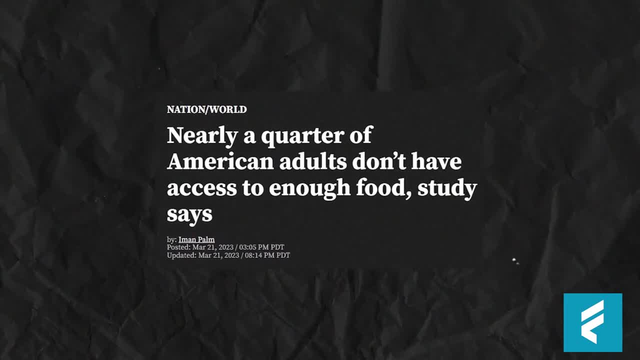 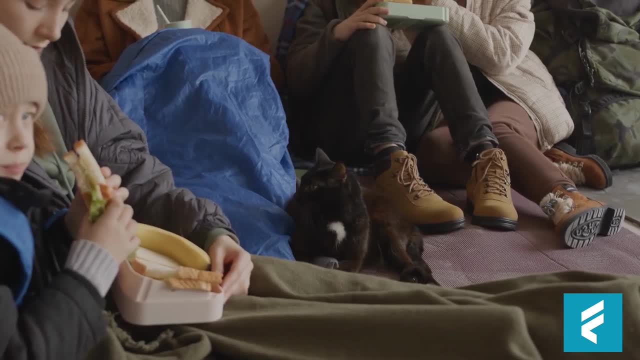 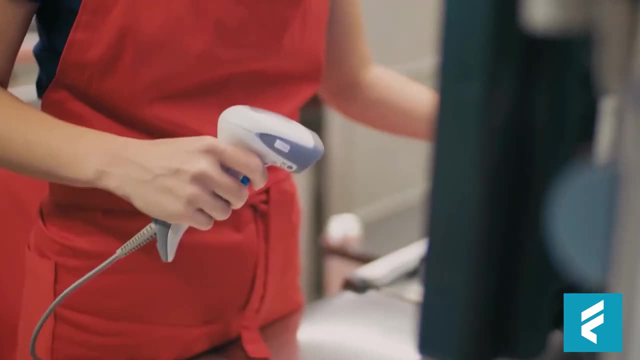 According to a recent study, almost 25% of American adults are currently experiencing food insecurity. This is a significant increase of approximately 5 percentage points from just a year earlier. The combination of rising inflation and the end of pandemic benefits has resulted in tighter household budgets, making it difficult for many families to put food on the table. 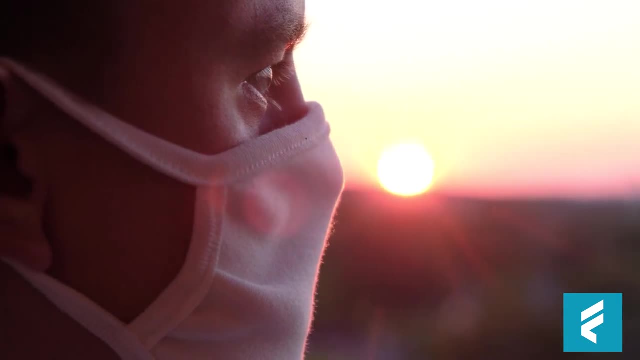 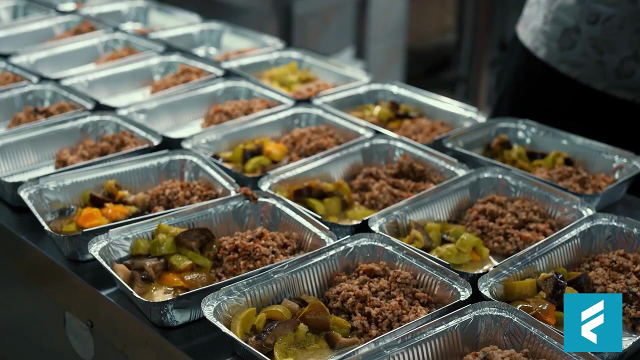 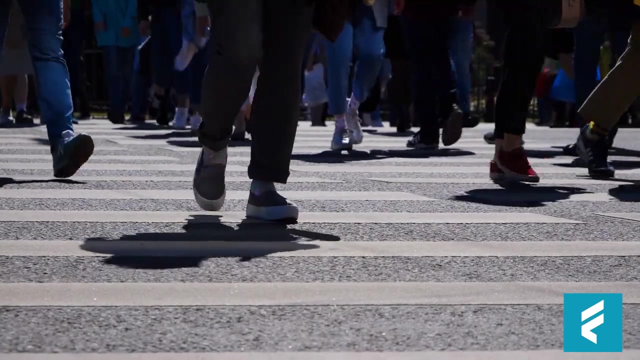 Food insecurity is a critical issue that affects millions of Americans each year. Defined as the ability to consistently access or afford adequate food, food insecurity has a far-reaching impact on individuals, families and communities. In addition to causing physical and mental health problems, food insecurity can also: 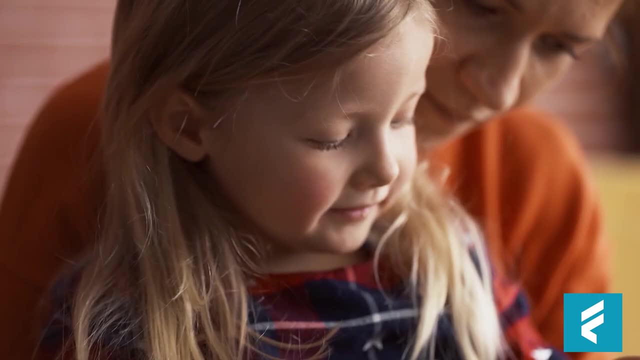 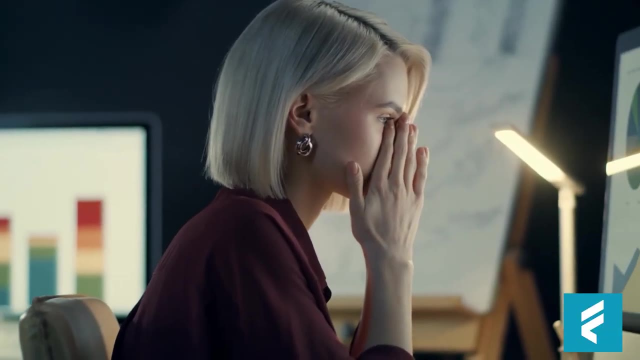 result in poor academic performance and reduced economic productivity. The current situation is particularly concerning because it reflects a significant increase in food insecurity rates in just a short amount of time. This suggests that the economic impact of the pandemic will have a significant impact on people's health and well-being. 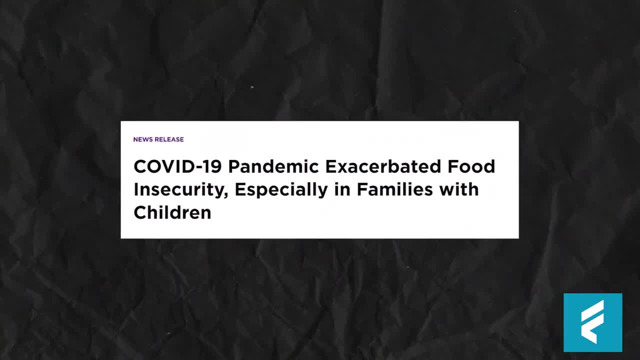 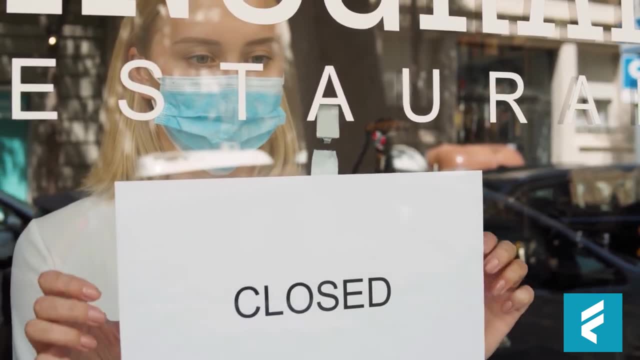 Food insecurity has become a rising concern for a significant number of American households. While government programs such as food assistance programs and unemployment benefits can help, it's clear that more needs to be done to address this issue. Food insecurity has become a rising concern for a significant number of American households. 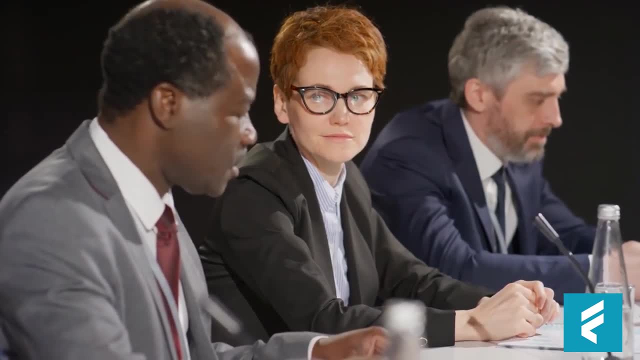 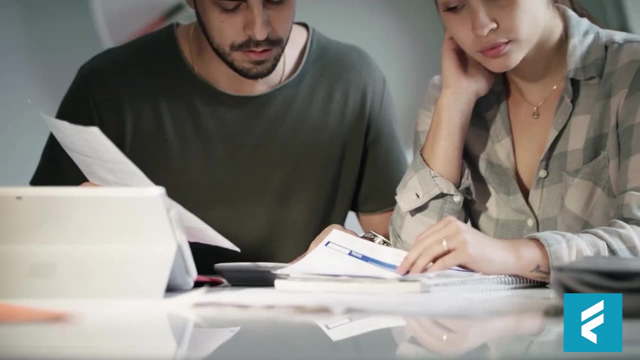 It is an alarming situation that indicates an inability to secure enough food for a nutritious diet. Such a situation can force individuals to skip meals or cut back on food intake, which can have severe implications on their health and well-being. Experts warn that this issue 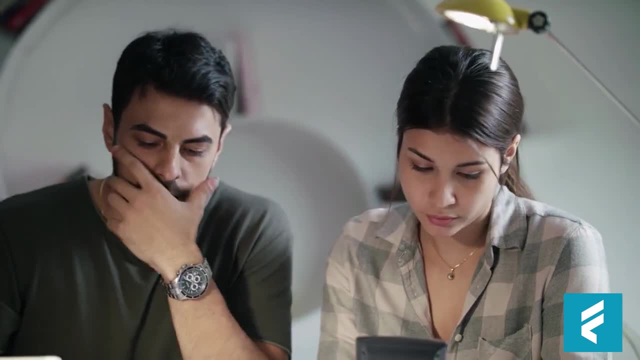 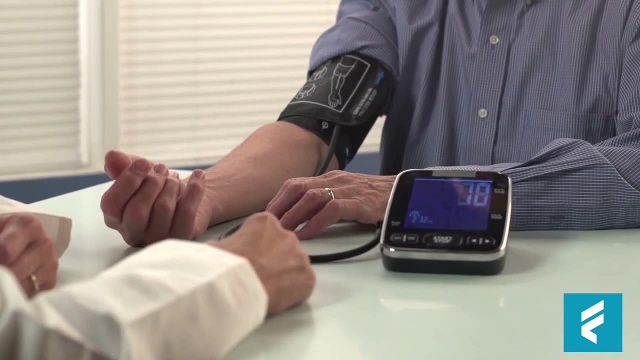 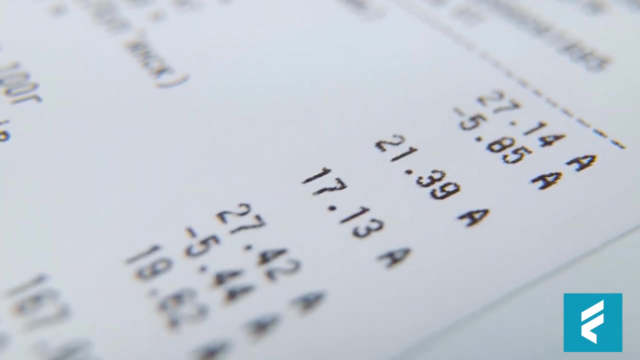 can contribute to malnutrition, chronic diseases and even mental health problems. The rise in food insecurity is attributed to the fact that more households are struggling to pay their typical bills. Grocery costs have surged by 20% in two years and rents have increased by 13%. The impact of these rising costs have been exacerbated. 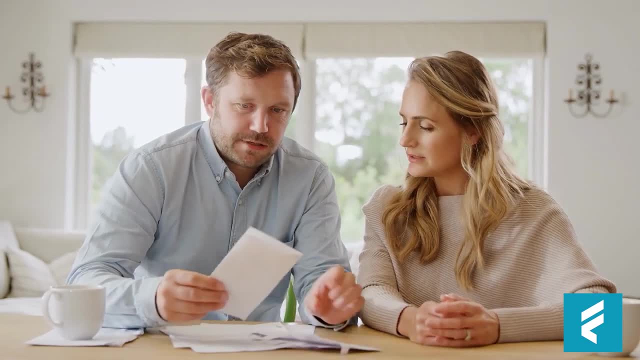 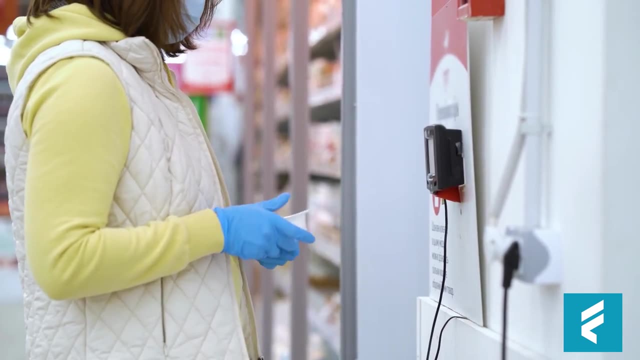 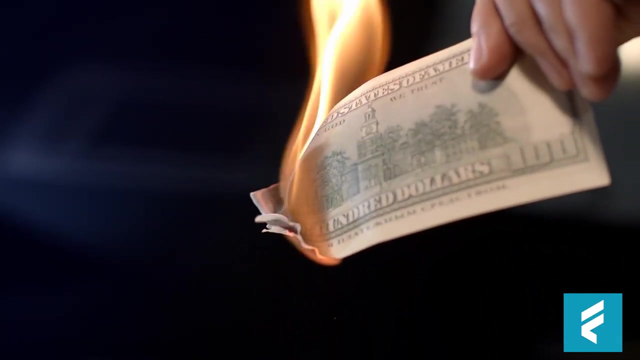 by inflation, which surged to a four-decade high last year. This double whammy of high inflation, inflation and the end of pandemic-related benefits has heightened the financial stress for many households, leading to a further increase in food insecurity. A new report from the Urban Institute reveals that almost 25% of American adults are food insecure. 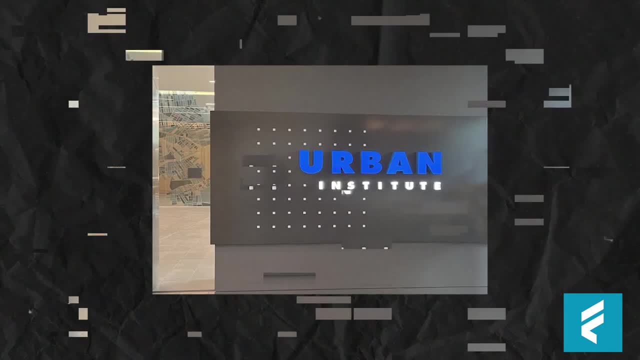 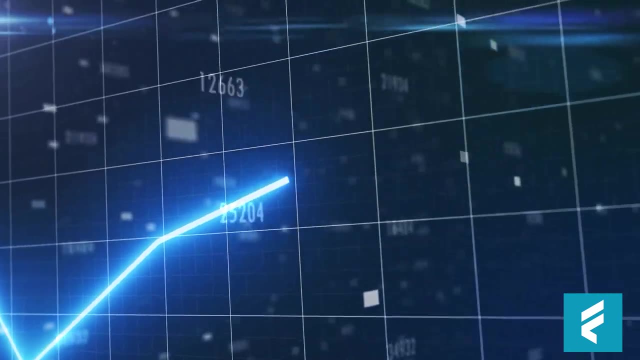 representing a jump of about five percentage points from a year earlier. The rise in food insecurity is a major concern and policymakers need to take immediate action to address it. The report highlights the importance of making food assistance programs more accessible and affordable. The report highlights the importance of making food 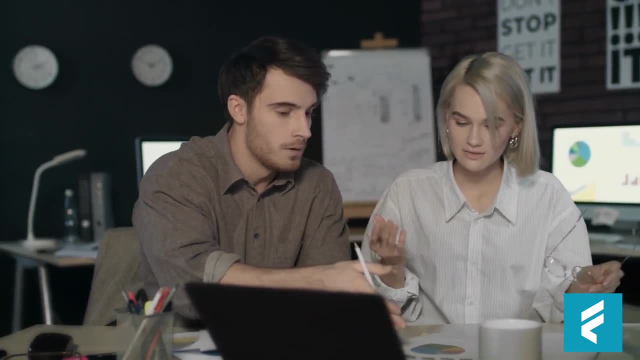 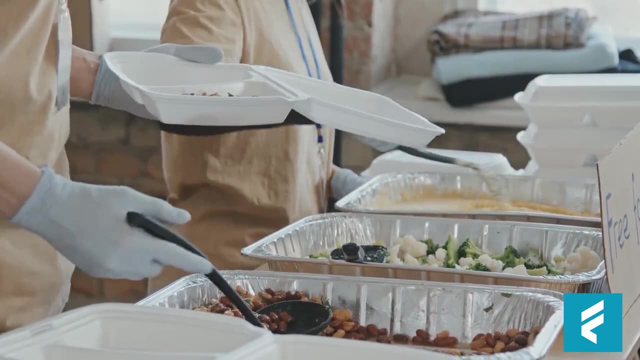 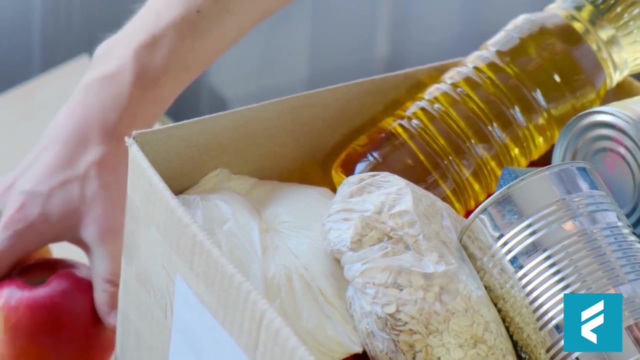 accessible and affordable, and expanding them to reach more households in need. It is evident that food insecurity is a complex issue that requires a multifaceted solution. Efforts should be made to address the root causes of this issue, such as poverty and income inequality. Additionally, it's crucial to invest in education and training programs. 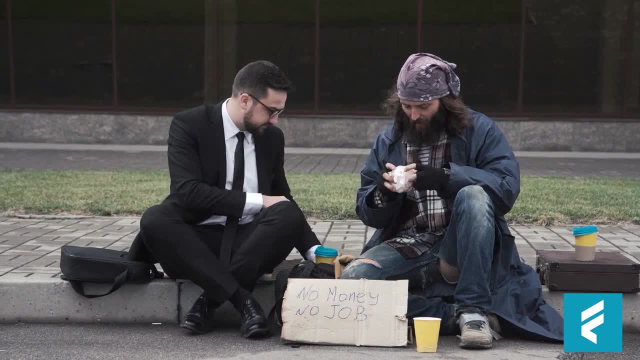 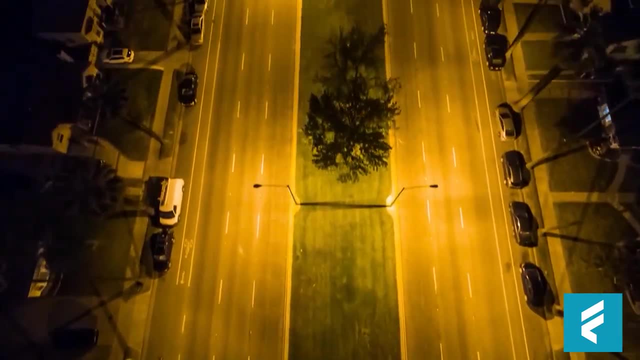 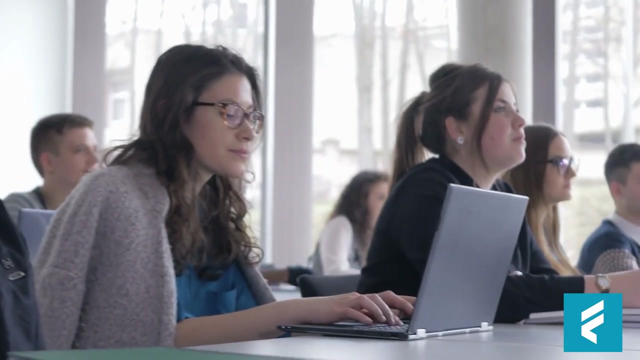 that can help individuals secure better-paying jobs and improve their financial stability. Ultimately, addressing food insecurity requires a concerting effort from all levels of society, including government, non-profit organizations and individuals, to ensure that everyone has access to nutritious food. Food insecurity has been identified as a red flag for households. 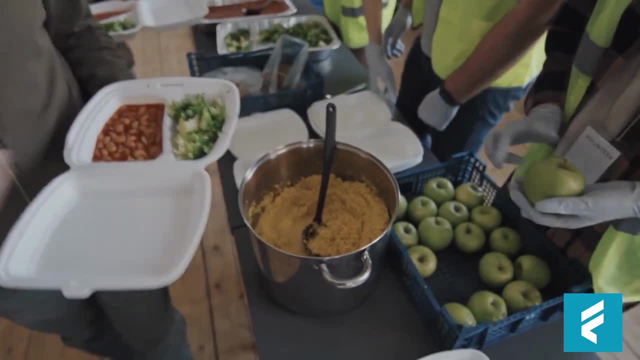 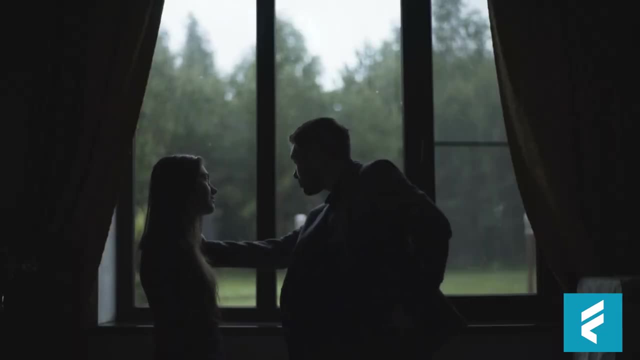 experiencing high levels of financial distress and the inability to meet basic household needs, as Kassandra Martynczak, a research associate in the Center on Labor, Human Services and Population at the Urban Institute, notes. Martynczak emphasizes that food insecurity is a household. 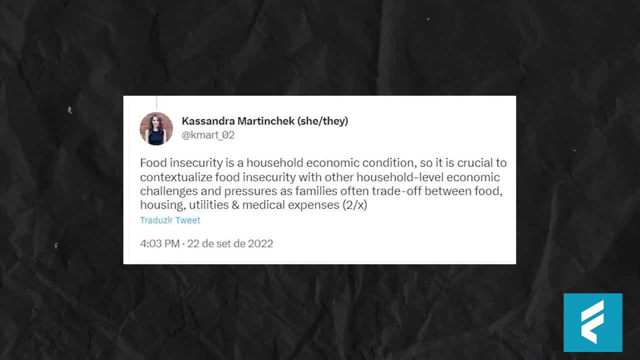 economic condition that leaves people with insufficient income and financial stability. Food insecurity is an economic condition that leaves people with insufficient income and financial stability. Food insecurity is an economic condition that leaves people with insufficient resources to acquire enough food for their families to lead active and healthy lives. 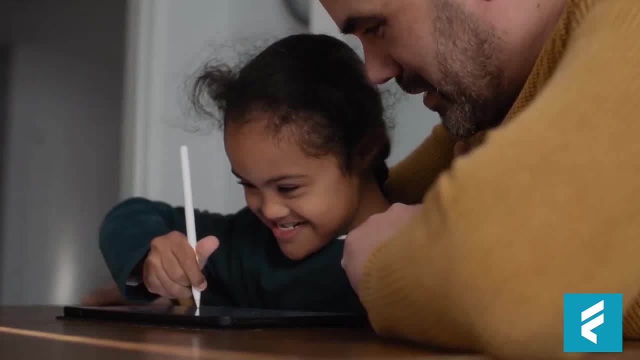 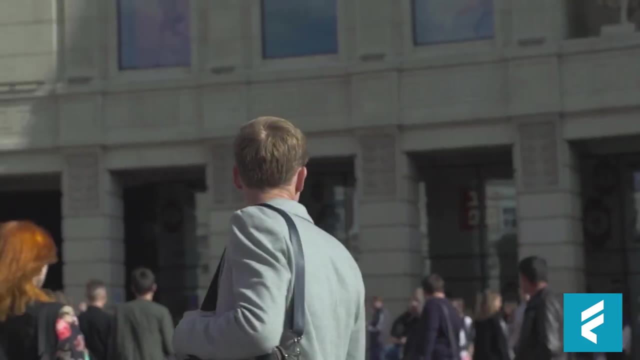 According to a new study by the Urban Institute, based on a survey of almost 8,000 adults conducted in December, almost 25% of American adults are food insecure. The figure represents a significant increase of about 5 percentage points from the previous year. as household, 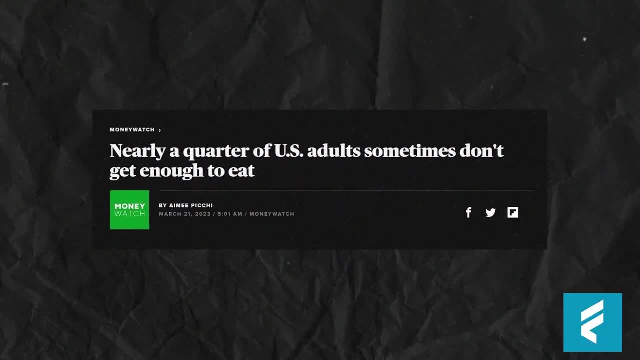 budgets continue to be squeezed by the double whammy of high inflation and the end of pandemic benefits. Moreover, the study reveals that one in six adults were likely to have food insecurity in their lives. This is a significant increase in the number of adults who relied on charitable food. 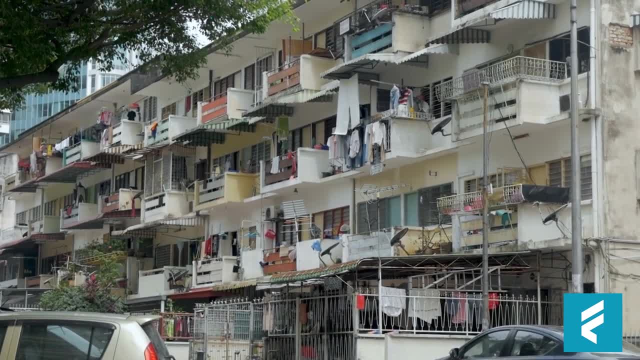 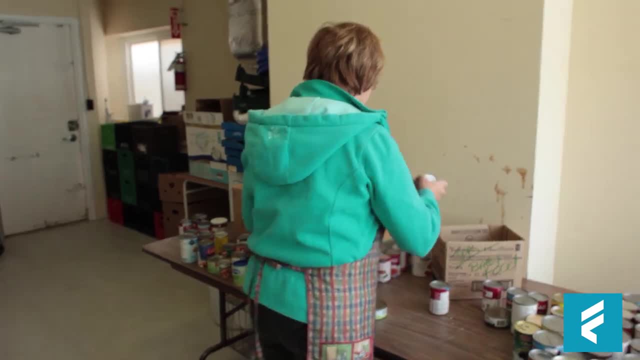 such as free groceries or meals in 2021.. This number represents an increase from the one in eight adults who relied on food charity in 2019, before the pandemic. The report highlights that food insecurity has implications for a person's health and well-being, as individuals resort to. 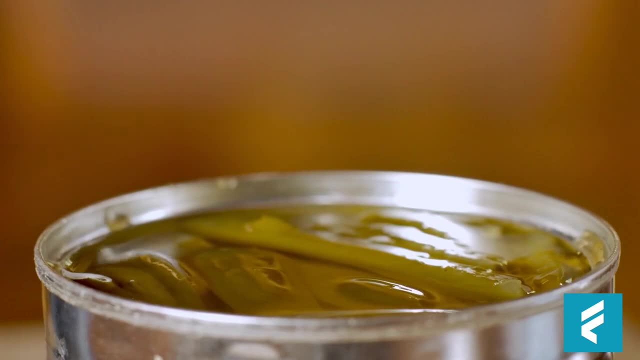 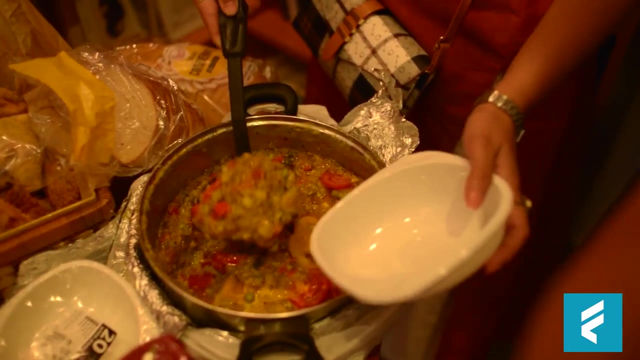 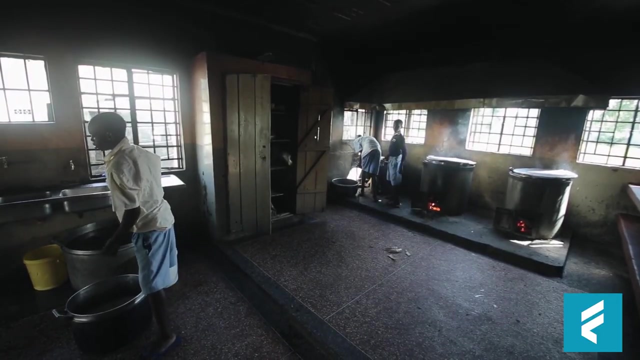 skipping meals or cutting back on food to cope with their situation. The rise in food insecurity is linked to the challenges faced by households in meeting their basic needs, as grocery costs surge- 20% in two years- and rents increased by 13% Inflation, which hit a four-decade high last year. 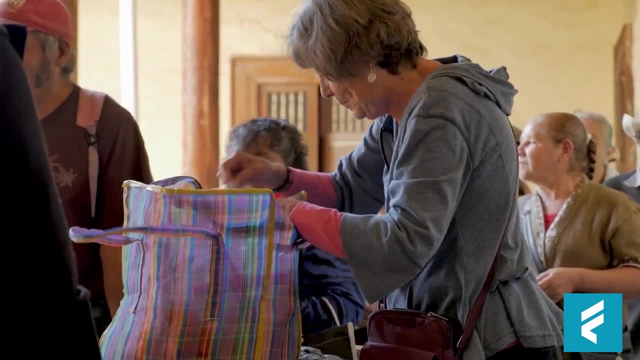 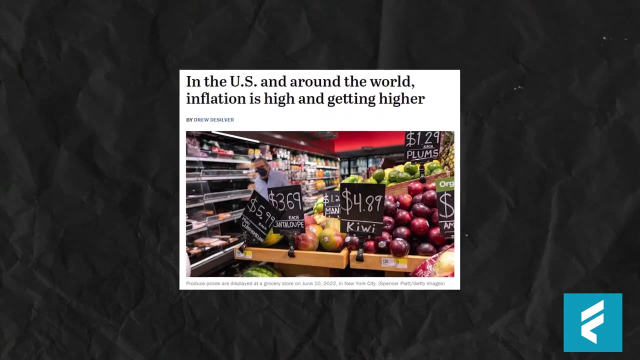 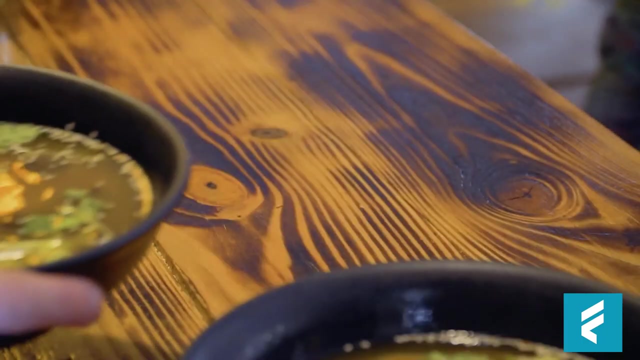 also compounded the financial stress for many families, particularly as several pandemic-related benefits came to an end. Despite a strong labor market, wages are not keeping up with inflation, which is eating into household purchasing power. According to the most recent data available, food stamp enrollment remains high, with 42.6 million people receiving benefits as of December. 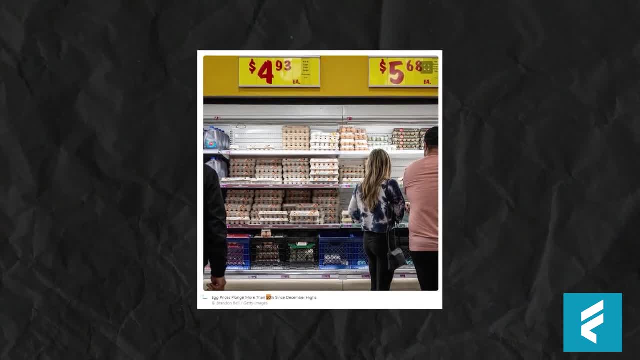 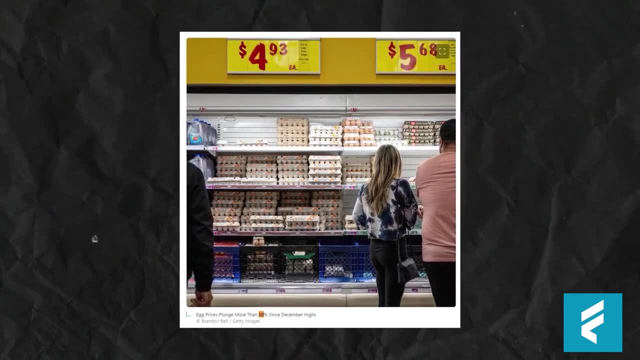 This is a significant increase in the number of adults who relied on food security in 2019 before the pandemic, highlighting the ongoing struggles of many households to meet their basic needs. The decision to prioritize one basic need over another can have a profound impact on the 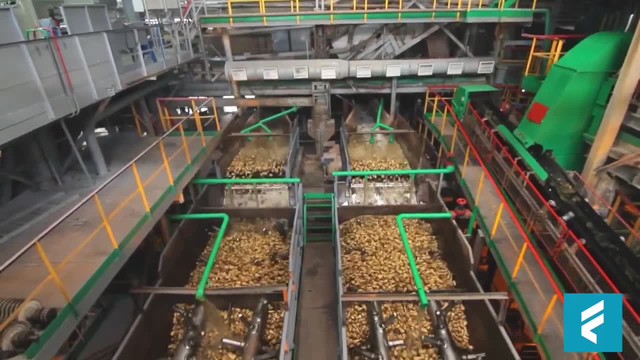 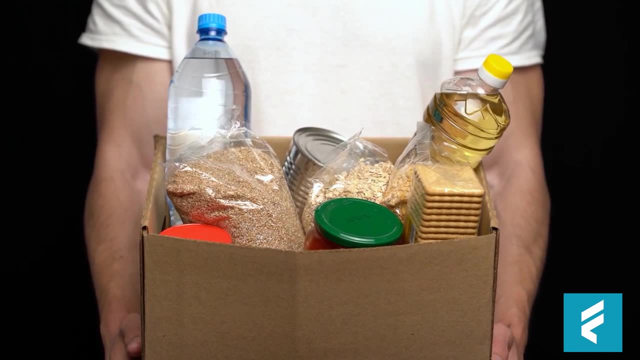 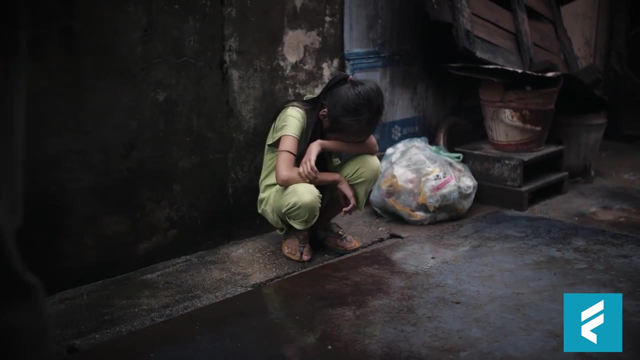 lives of those who are food insecure. Families may have to choose between putting a roof over their heads or putting food on the table, or between buying necessary medication or purchasing groceries. These tough decisions can lead to negative consequences on a person's health and well-being. according to experts, Food insecurity is a growing concern in the United States. 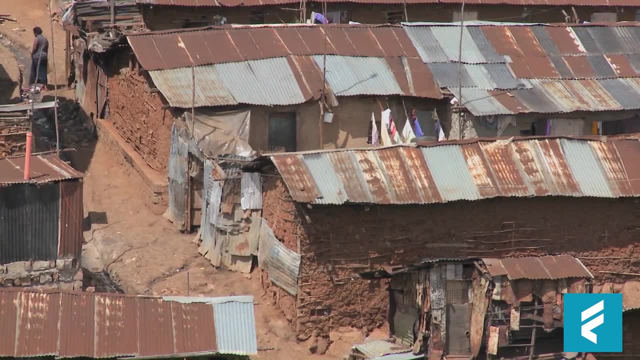 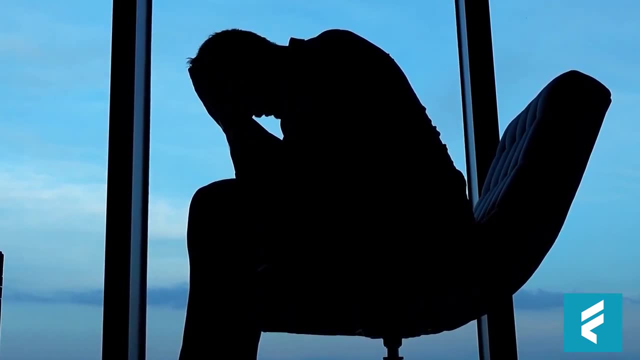 with nearly 25% of American adults struggling to secure enough food for a nutritious diet, a jump of about five percentage points from the previous year, according to a new report from the Urban Institute. The rise in food insecurity comes amid a surge in grocery costs, which have 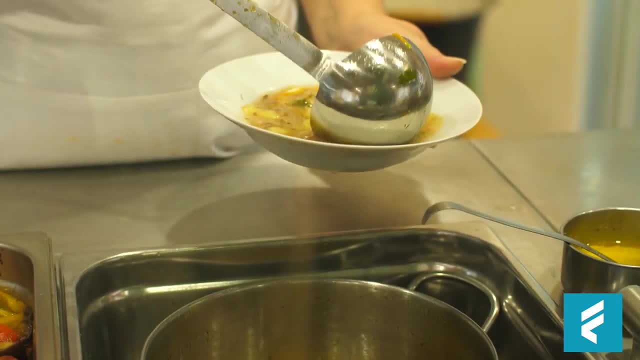 increased by 20% in two years and 13% increase in rent. Inflation also surged to a four-decade high, just as several pandemic-related benefits have increased. The rise in food insecurity has also increased in the United States, with nearly 25% of American households struggling to secure enough. food for a nutritious diet. In addition, the rise in food insecurity has increased in the United States, which has increased by 20% in two years and 13% in two years. The rise in food insecurity has also increased in the United States, which has increased in the United States, and the increase in food 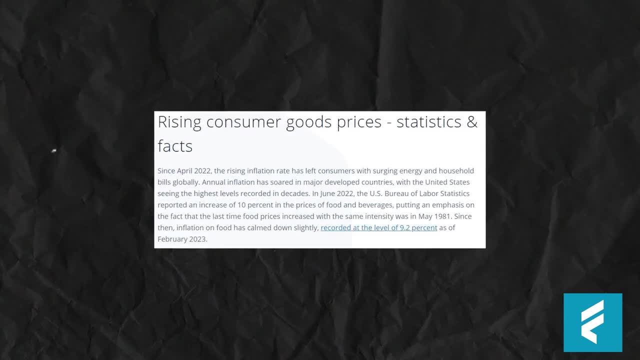 insecurity has increased in the United States, which has increased in the United States, heightening the financial stress for many households. The study, based on a survey of almost 8,000 adults in December, found that about 1 in 6 adults 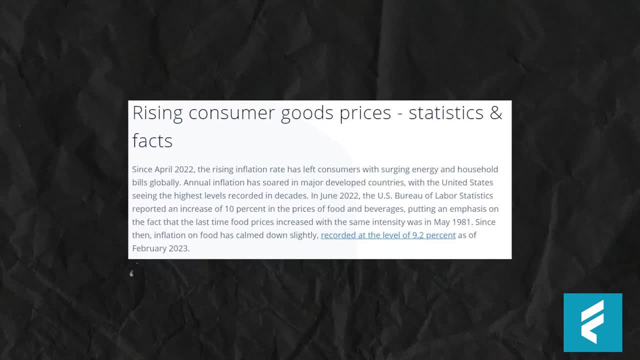 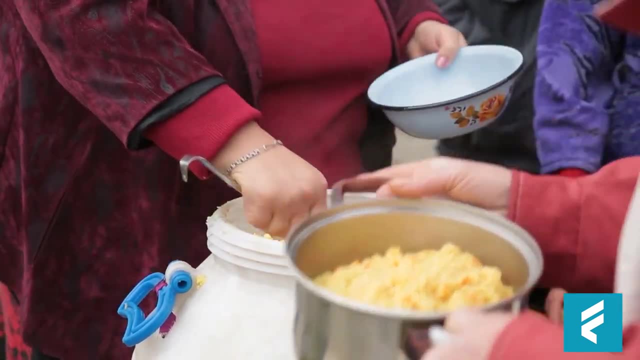 relied on charitable food, such as free groceries or meals last year, compared to 1 in 8 adults who relied on food charity in 2019, prior to the pandemic. Furthermore, despite more Americans finding jobs and the labor market remaining strong, wages are not keeping up with inflation. 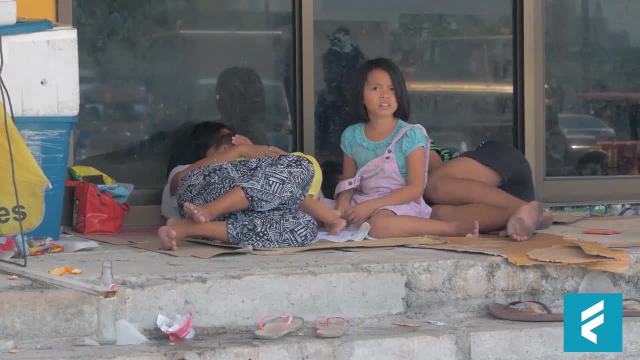 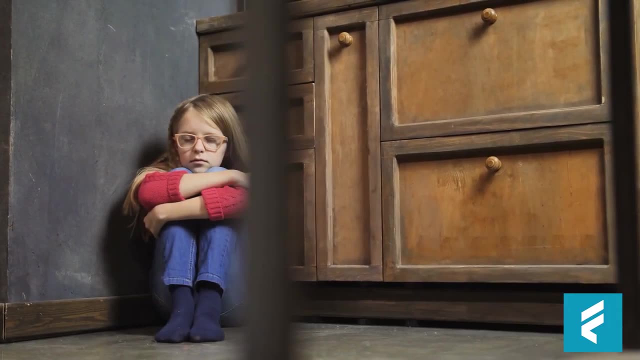 chipping away at household purchasing power. Food stamp enrollment also remains high, with 42.6 million people receiving benefits as of December, which is about 15% higher than prior to the pandemic. Moreover, the impact of high grocery costs is felt disproportionately by those who were 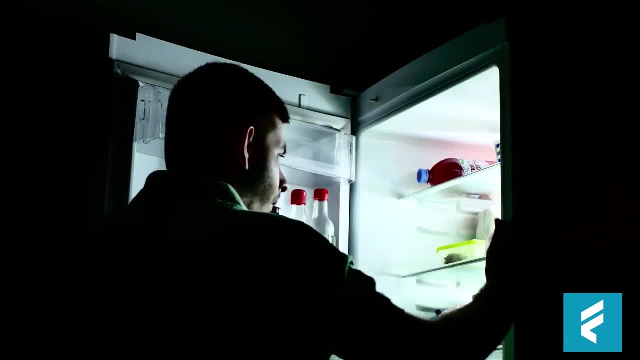 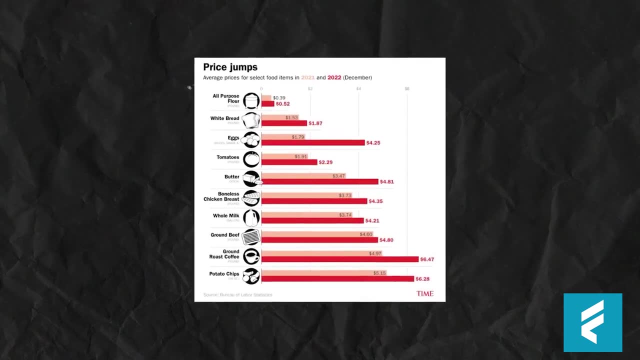 already struggling to make ends meet. Adults whose grocery costs increased a lot in the last year were about twice as likely to be food insecure compared to other adults. This can lead to a cycle of poverty that is hard to break out of as food insecurity. 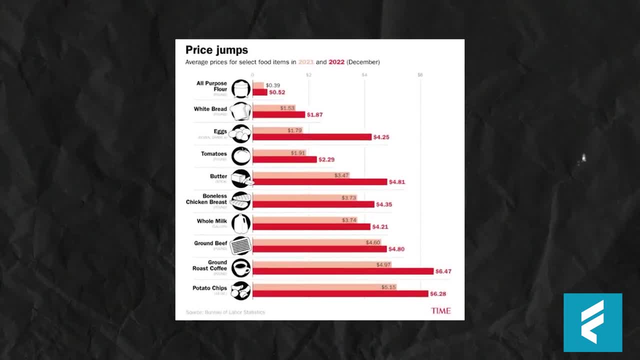 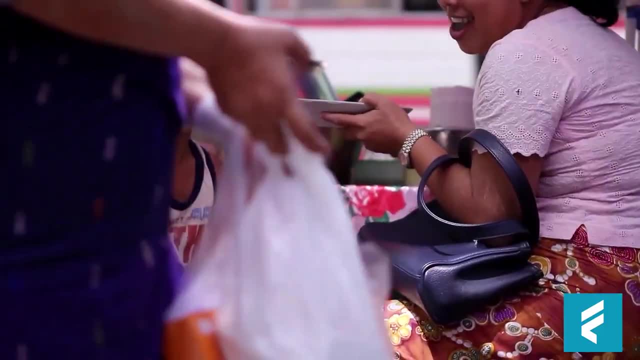 can exacerbate health problems and can lead to job loss or an inability to work. In the face of these challenges, experts stress the need for solutions to address food insecurity in America. This includes increasing access to affordable, nutritious food through programs such as SNAP. 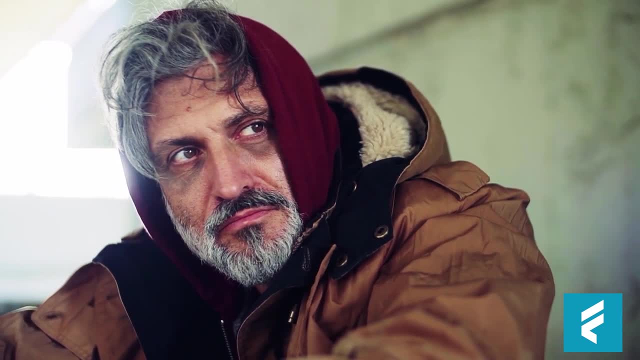 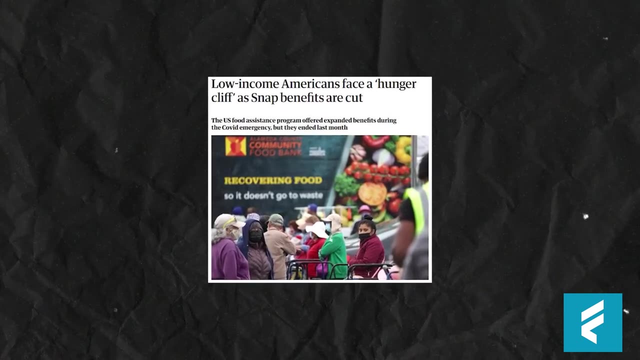 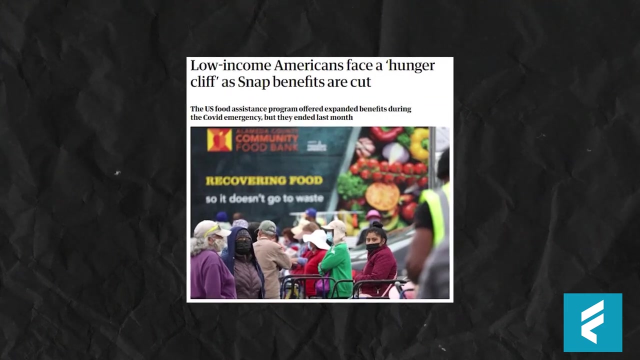 and expanding food bank and food pantry services. It also involves addressing the root causes of poverty and income inequality, which can create conditions that are difficult to deal with. Ultimately, addressing food insecurity is a complex issue that requires coordinated efforts across multiple sectors to ensure that everyone has access to the food they 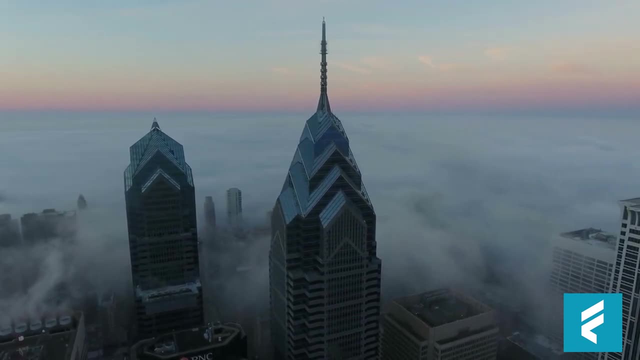 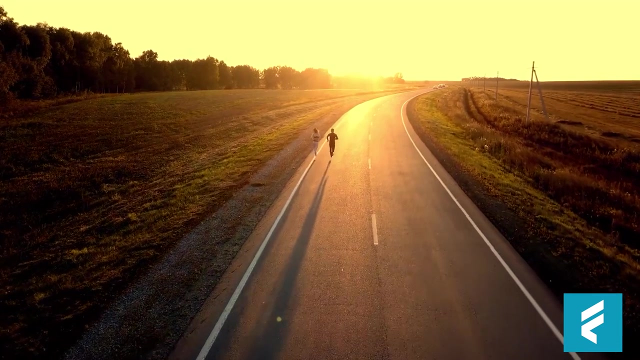 need to live healthy, fulfilling lives. Food insecurity is a persistent problem in the United States, affecting millions of individuals and households each year. The recent report from the Urban Institute highlights how the pandemic inflation and the end of pandemic benefits have exacerbated the situation for many. 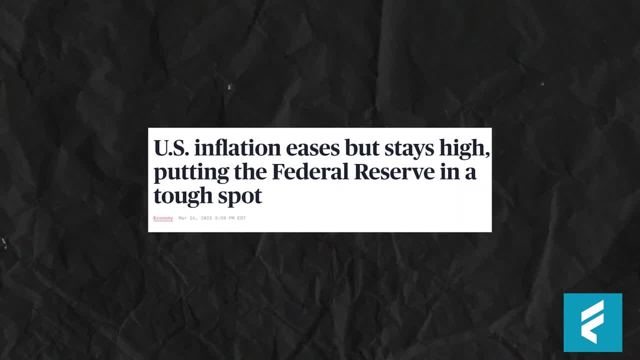 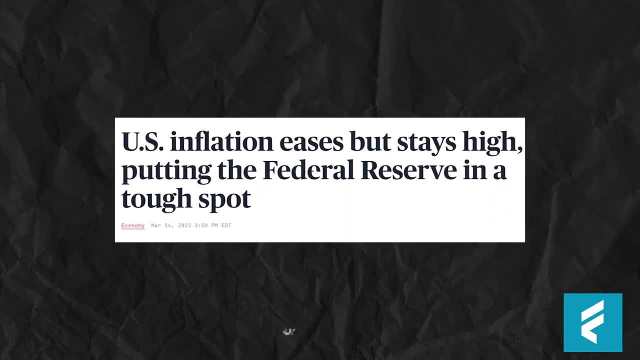 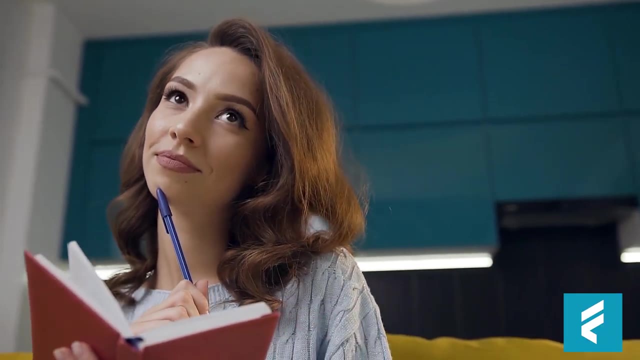 According to Cassandra Martynczak, a research associate in the Center on Labor, Human Services and Population at the Urban Institute, food insecurity can be a sign of deeper economic struggles. In households experiencing high levels of hardship, it can be difficult to make ends. meet and secure enough food for a nutritious diet. The situation is made worse by the fact that grocery costs have surged by 20% in the last two years, While rents have increased by 13% in the last two years. food insecurity has also increased.